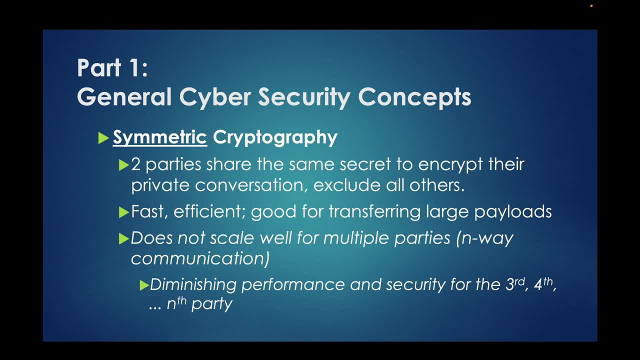 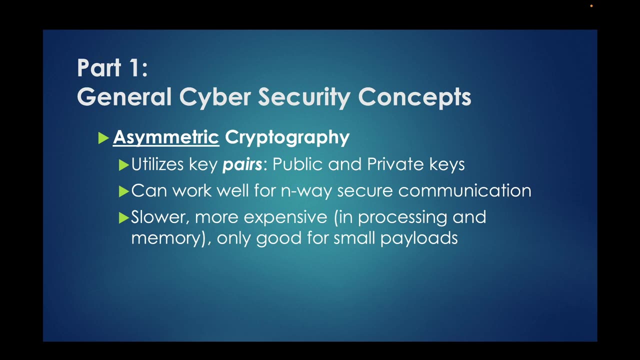 by direct communication, by email, text, USB stick or carrier pigeon, which reduces efficiency and security with each additional party. Asymmetric cryptography, instead of sharing one key, utilizes key pairs in a special scheme: public and private keys, Because the public key is just that public and because the private key is just 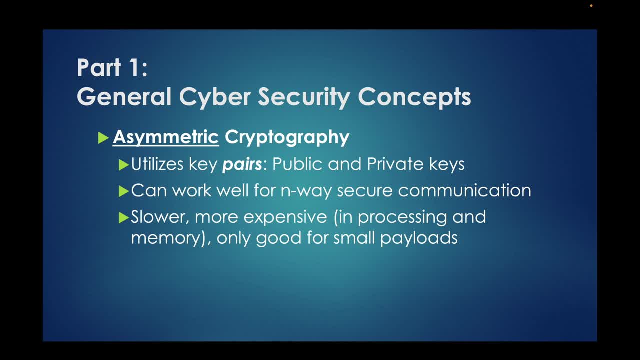 just that, never shared. there are no logistical issues of securely delivering a secret key to the next party to the conversation. As such, asymmetric key cryptography is well suited to n-way communication. That being said, when compared to symmetric key cryptography, asymmetric is slower, more expensive in terms of processing and memory resources. 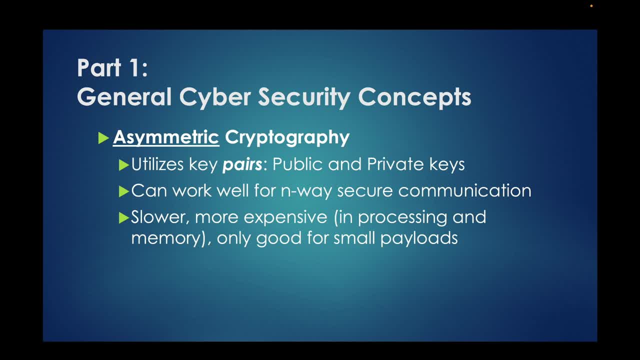 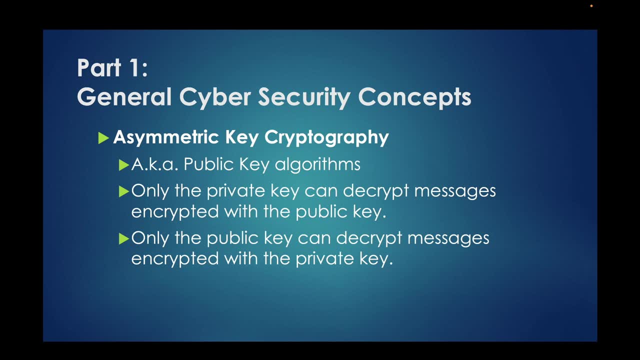 and only suited for exchanging small quantities of data at a time. Here, at a high level, is how the magic works. The public and private keys are mathematically related. Only the private key may decrypt messages encrypted with the public key, And only the public key may decrypt messages encrypted with the private key. 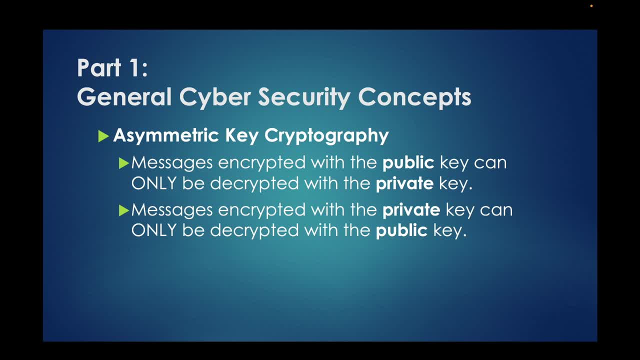 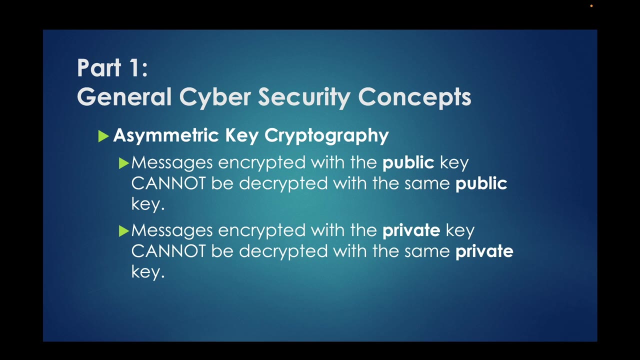 Put another way: messages encrypted with the public key can only be decrypted with the private key, And messages encrypted with the private key may only be decrypted with the public key, And the corollary is that messages encrypted with the public key cannot be decrypted with the same public key. 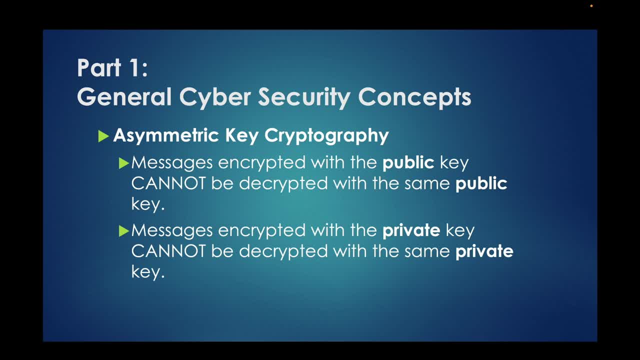 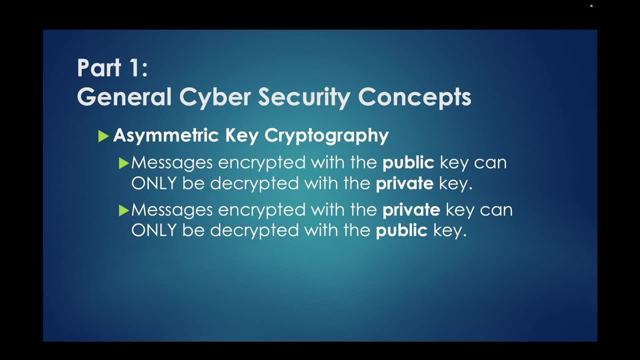 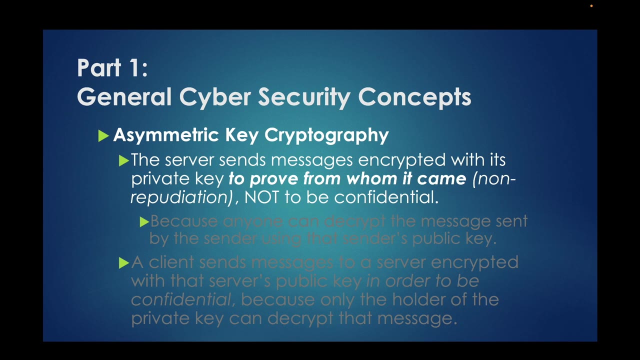 And messages encrypted with the private key cannot be decrypted with the same private key. I stated that three different ways, just to be certain you are completely clear on the concept of public and private keys. A server sends messages encrypted with its private key to prove from whom it came. 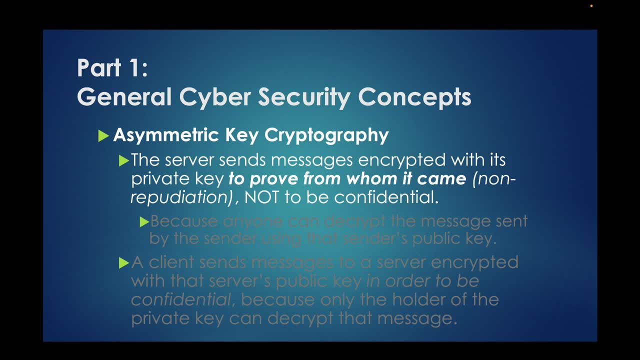 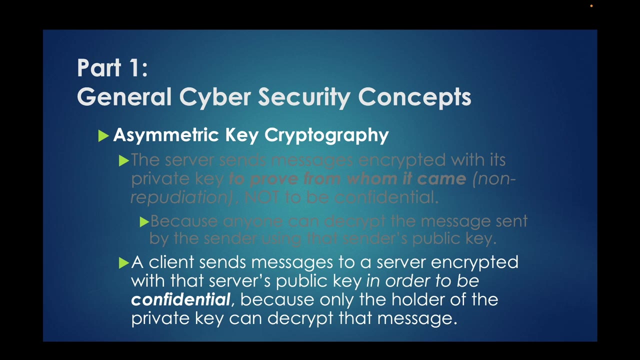 which is non-repudiation not to be confidential. The message is not confidential because anyone may decrypt the message sent by the sender using that sender's public key. A client sends messages to a server encrypted with that server's public key in order to be confidential. 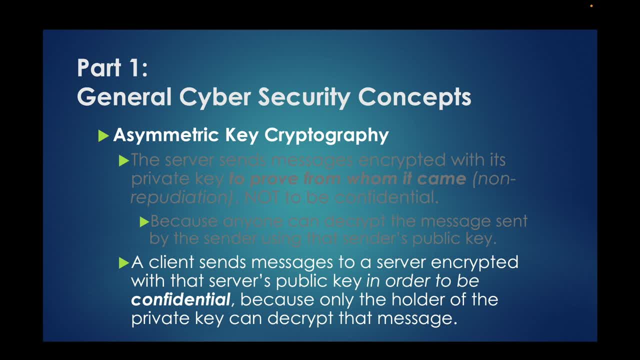 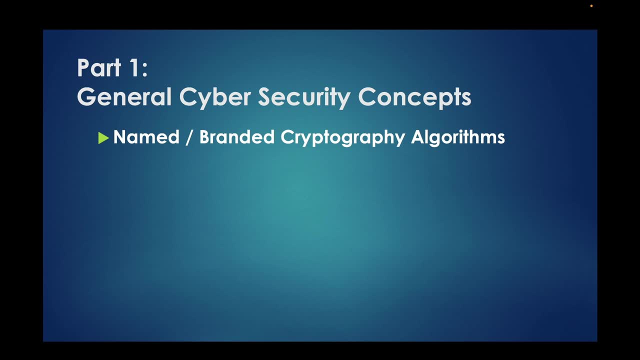 because only the holder of the private key may decrypt that message. Now that we understand symmetric and asymmetric, or public and private key cryptography, let's learn something about the named or branded algorithms for these purposes. Next,